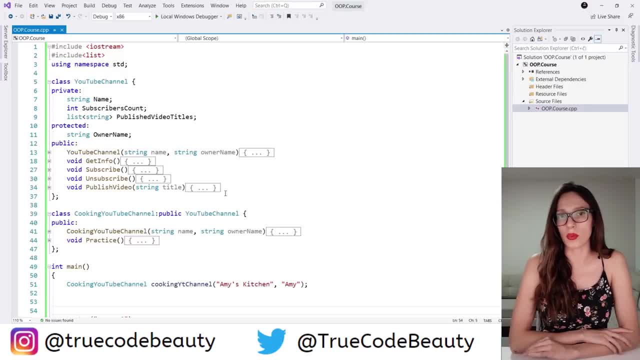 polymorphism. Now, the first thing that I want to do is I want to explain what is polymorphism. Polymorphism describes the ability of an object, for example, to have multiple forms. Now that means that you can have two or more objects that inherit from the same base. class Those objects. 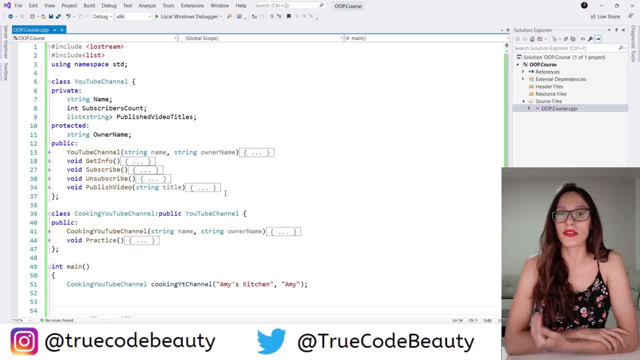 can have the method that has the same name, but different implementation, meaning different behavior, And I'm going to demonstrate that on an example. Now, here I have some code that we have written in my program And I'm going to demonstrate that on an example. Now, here I have. 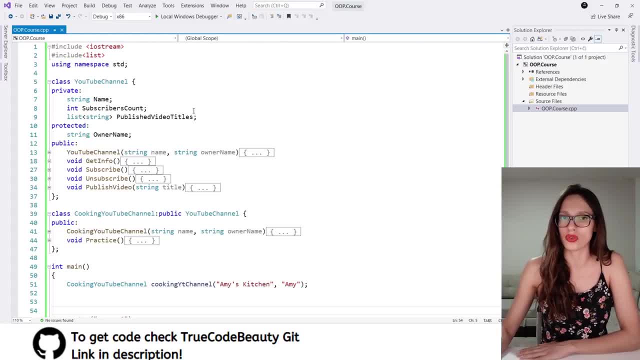 previous courses, so if you haven't watched those, make sure to do so. The links to those videos are going to be in the description, And I'm very quickly going to go over this code. So here I have created a class that is called YouTube Channel. That class has three private properties. 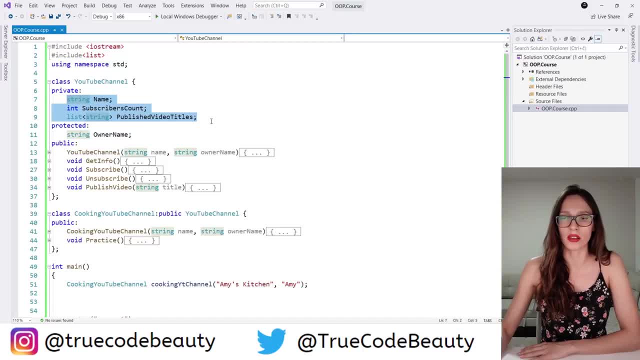 name, subscribers count, and then published video titles, And then it has one protected property which is owner name. Now these private properties, these are available only in this class. And then these protected properties, these are available in derived classes as well. And then here we have public. 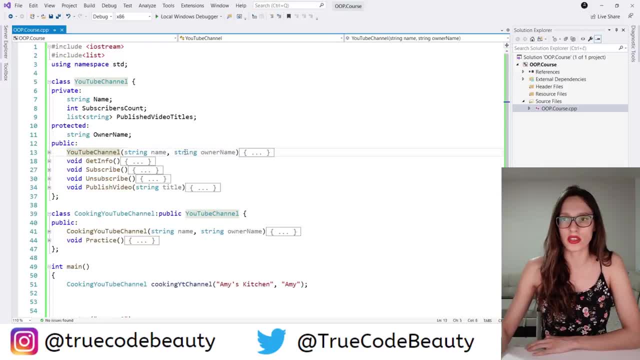 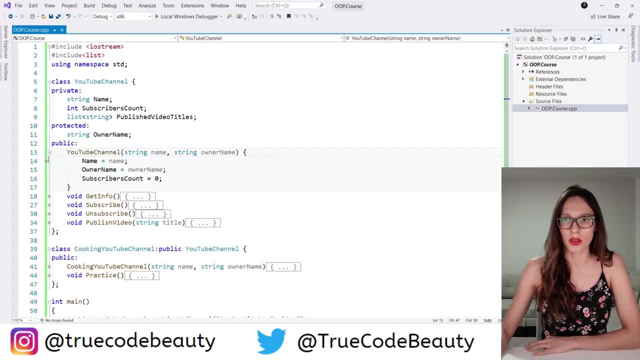 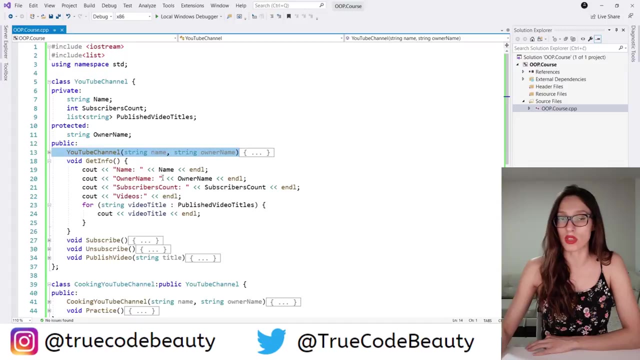 methods as well, And this here is our constructor, So it just initializes values of these properties. I'm going to collapse that. And then here we have get info method which just writes out information about the object. And then here we have get info method which just writes out: 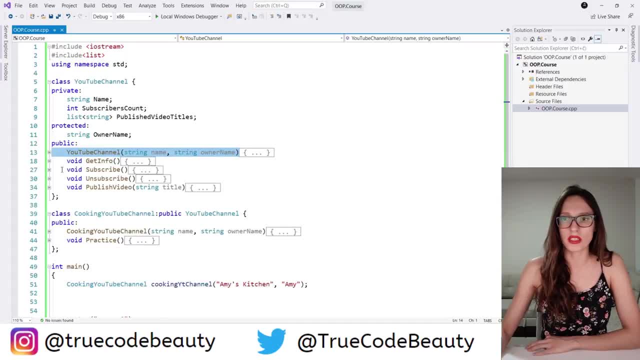 our YouTube channel And then these subscribe and unsubscribe methods. these just increase or decrease the number of our subscribers. Let's collapse that And then publish video method. it just adds another video to this published video titles list. So that would be our YouTube. 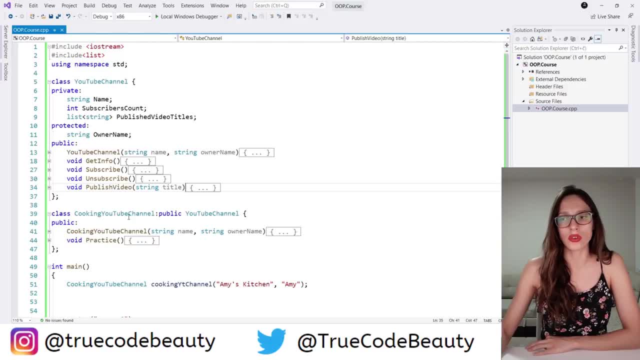 channel base class, And then here we have cooking YouTube channel, Which is a specific type of YouTube channel that inherits from this base class here And that cooking YouTube channel has its own constructor, which is this one. here And here we have just invoked the constructor of our base class, And then here we have implemented a method which is: 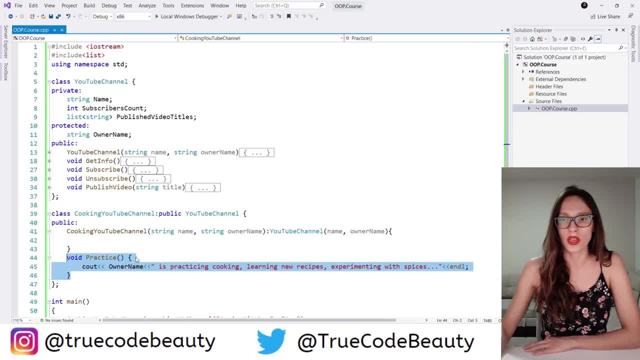 called practice And it says that when you practice and you have a cooking YouTube channel, you will have to be practicing cooking and then learning how to cook, And then you have to be practicing learning new recipes and experimenting with spices. Now, what I want to do is I want to create. 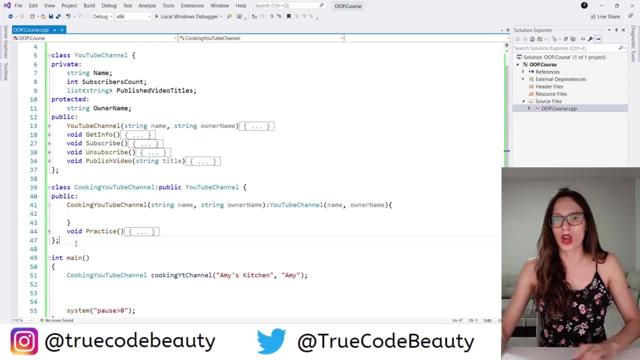 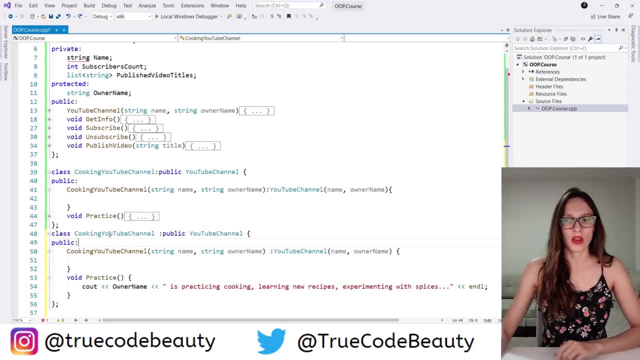 another derived class. So I'm going to copy this, Okay, And then this derived class should be called, for example: let's paste the name here: So singer's YouTube channel, And I'm going to paste the name here as well, on my constructor, So this is going to be a YouTube channel. 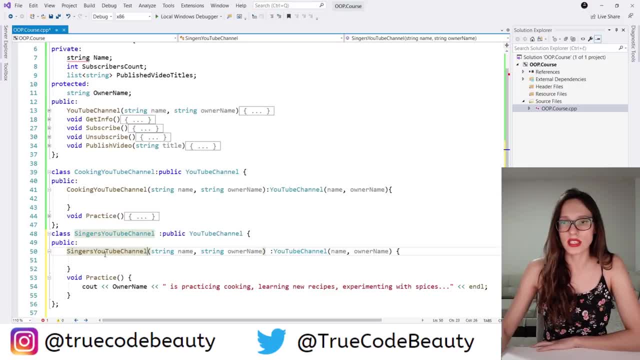 about singing now, as you can see, this singer's YouTube channel has this practice method as well, but this implementation is not right for my singers YouTube channel because if you're a singer, you are not going to benefit really from practicing cooking and then from learning recipes and 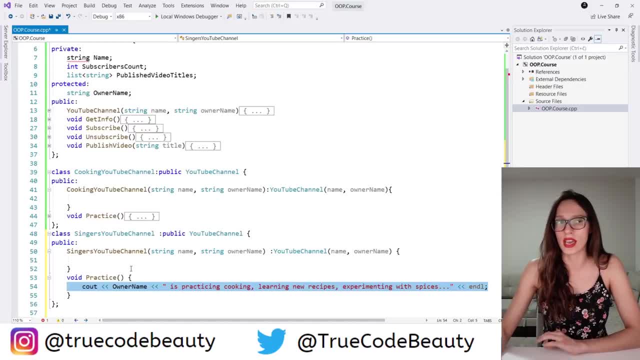 experimenting with spices, but what you should do instead is you should practice something else. so I'm going to copy that so that I don't make a typo like this. so someone who is trying to make a singers YouTube channel is going to take singing classes and then learning new songs, and then he should as well be. 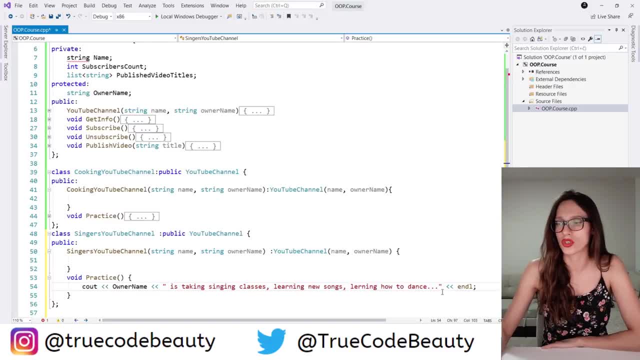 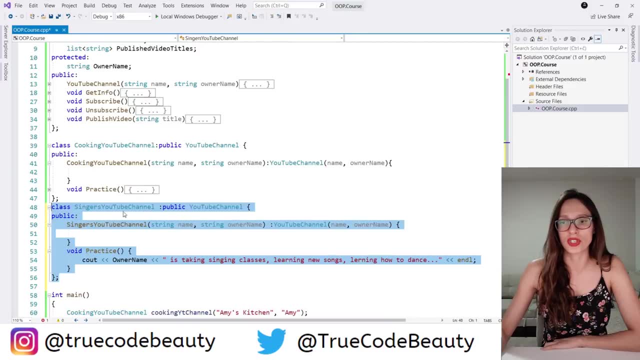 learning how to dance, because I believe that singers should know how to dance as well. okay, so now we have implemented this singers YouTube channel And, as you can see, as I already demonstrated, it has this same method, which is practice, but this method has different implementation than this one And, as you can see, 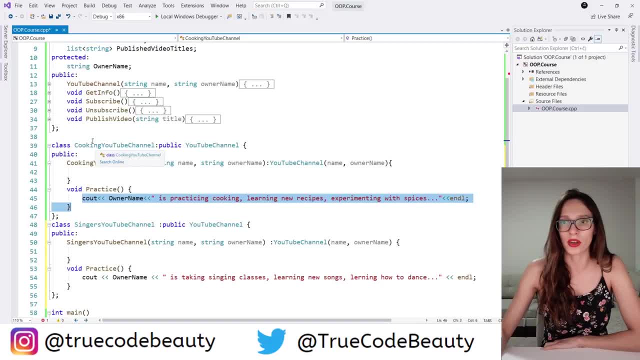 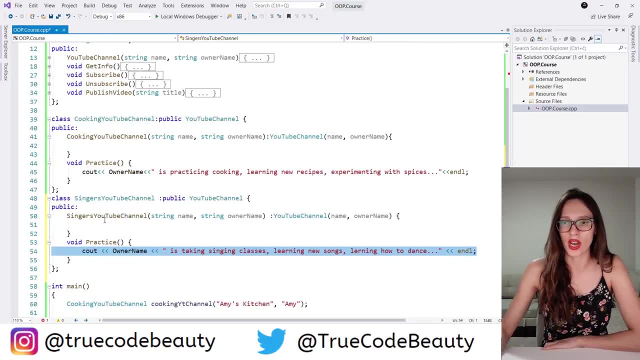 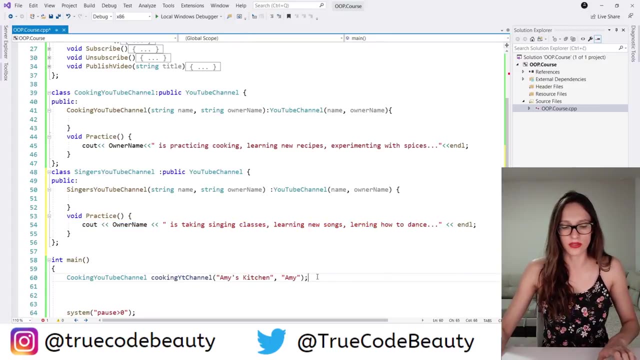 here. this is the implementation of our practice method on our cooking channel. And then this here is the implementation on our singers YouTube channel. So what I want to do now is I want to create this singers YouTube channel Here. we already have cooking YouTube channel, So it is a. 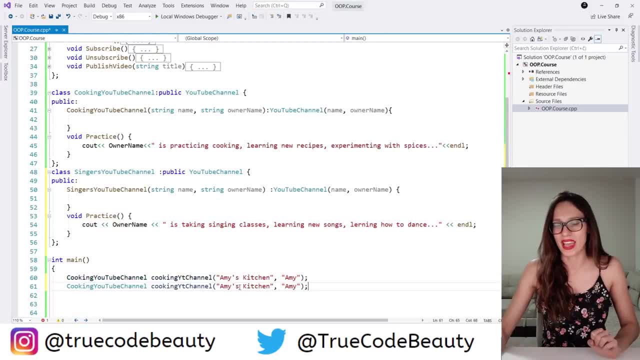 video. it is a code from one of my previous videos, And then what I want to do is I want to create singers YouTube channel. So let's call it singers YouTube channel, And let's say that it is going to be called. for example, John sings like this, And then owner is going to be a guy named John. 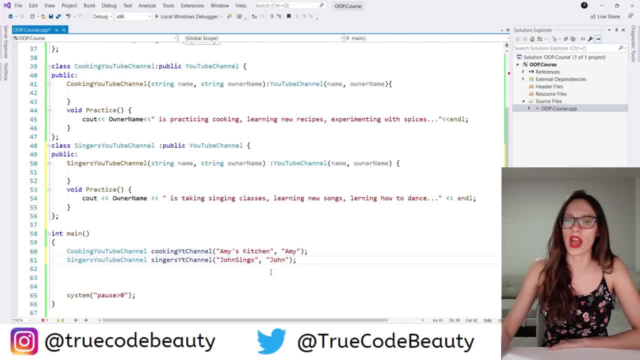 Like this: Okay, Now, after I have created this cooking YouTube channel and then this singers YouTube channel, you can probably call it singing YouTube channel or something like that. This is the best name that I could come up with. Okay, So now what I want to do is I want to invoke 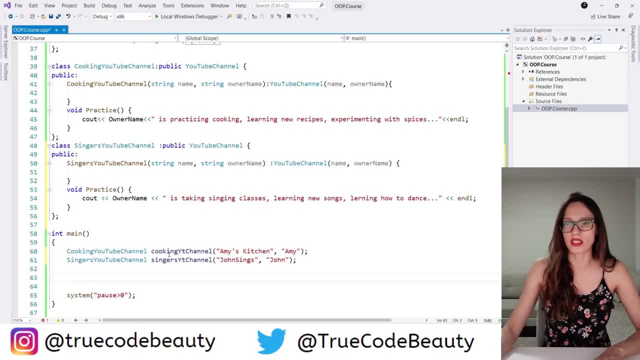 methods on these two classes, And the methods that I want to invoke are going to be these two. So practice, and then this practice method as well. So here I'm going to say cooking YouTube channel Practice like this, And then let's invoke the same. 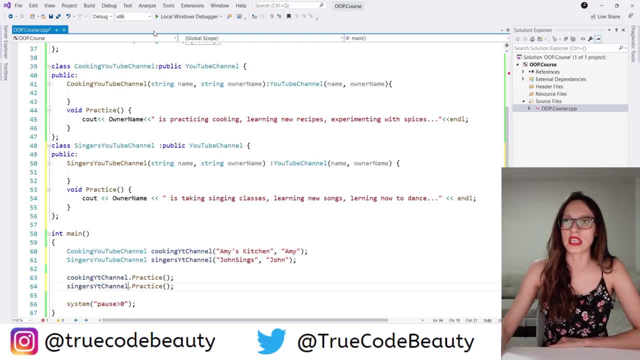 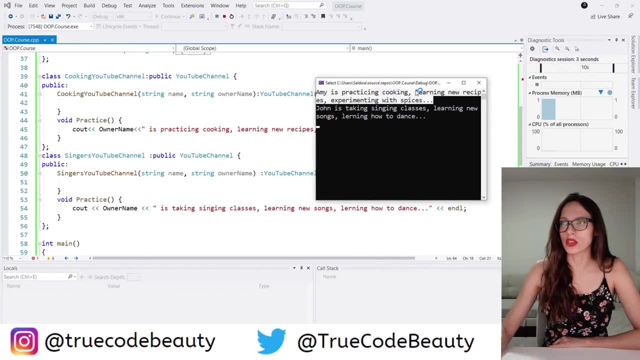 method for my singers YouTube channel Like this, And now, if I run my program, as you can see, it says that Amy is practicing cooking and then John is taking singing classes and learning new songs and learning how to dance. I can imagine that, Okay. 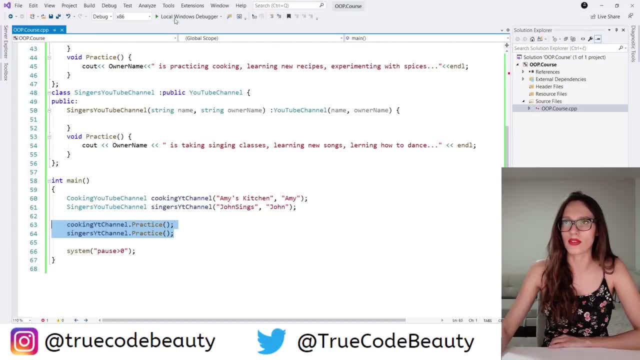 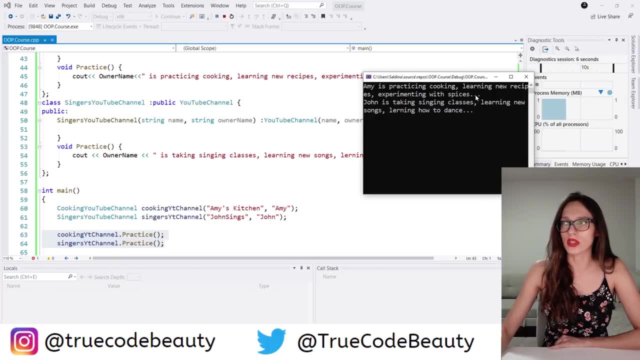 And then, after I have invoked these two methods, you can really see: oh, I have stopped my program, I'm sorry. So here you can see that this cooking YouTube channel has invoked its own method. So this cooking YouTube channel has invoked the method that has been implemented in this. 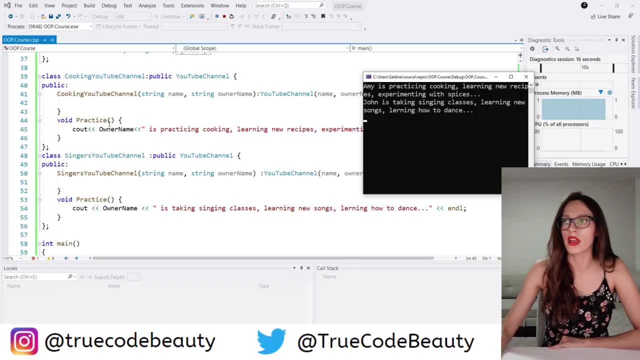 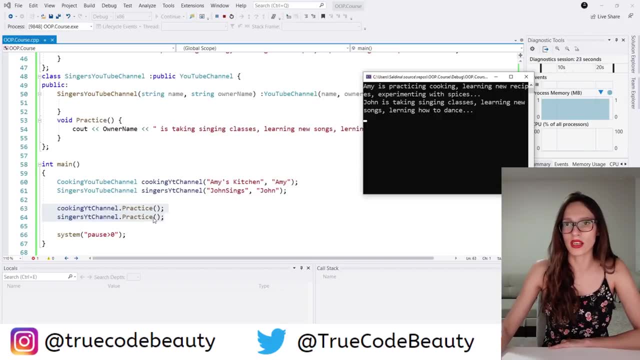 cooking YouTube channel class, which is this one here, And then this invocation: So this singers YouTube channel- when you invoke practice method on that, this method here is going to be invoked. So this method that is implemented in singers YouTube channel class. 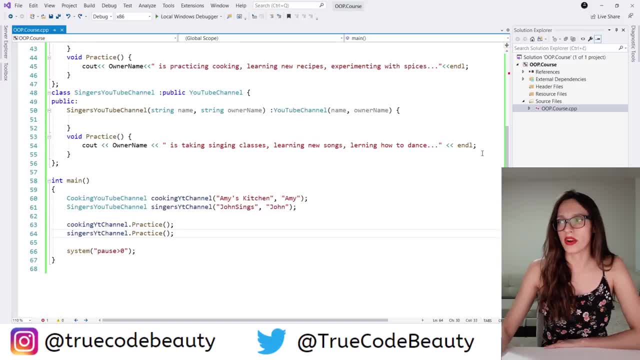 Now let's add another thing, And that is going to be here in this practice method, And then in this practice method as well. what I want to do is I want to say that each time that our user practices cooking and then practices singing, what is going to happen is the quality. 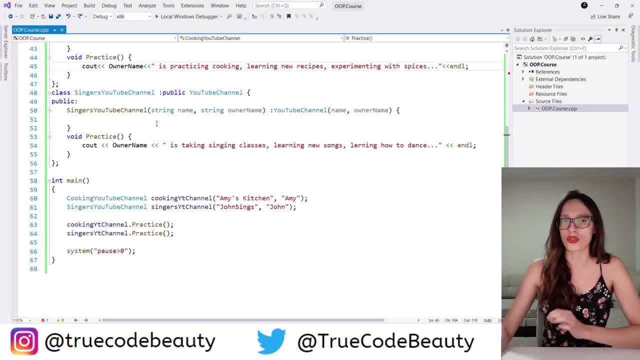 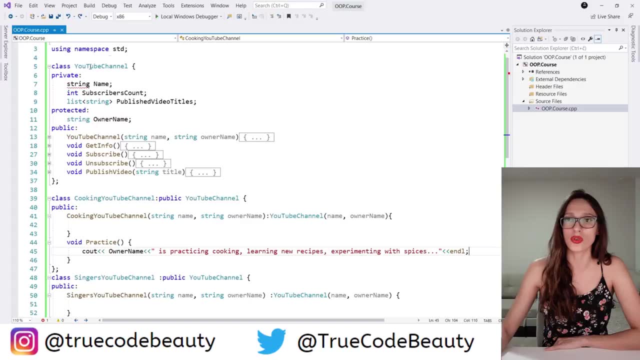 of that YouTube channel is going to increase. So in order to track that quality content rating, I'm going to create a property and that is going to be here in this YouTube channel in this base class. So I'm going to make that property protected because I 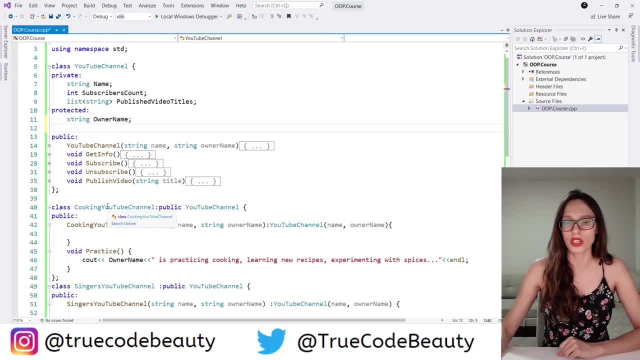 want to have it accessible in my cooking YouTube channel and then in my singers YouTube channel as well. So I want that property to, I want to access that property from my derived classes And because of that I'm going to make it protected. So here I'm going to say int and 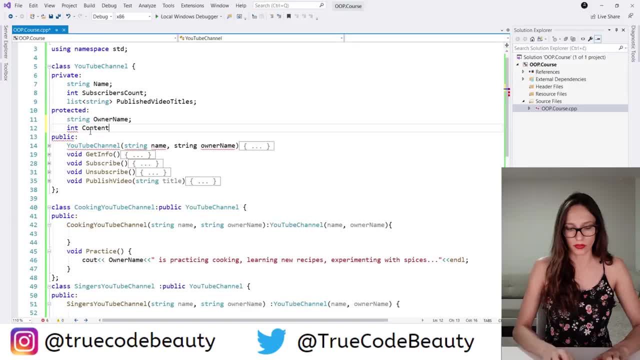 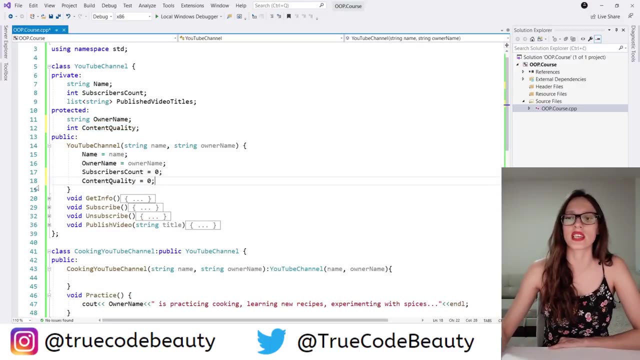 let's call it content quality, Like this. Okay, And initially, I want to set the value of this content quality variable in this constructor here. I want to set it to zero, like this, because I want to say that when you create your YouTube channel, this constructor here is going to be invoked, and 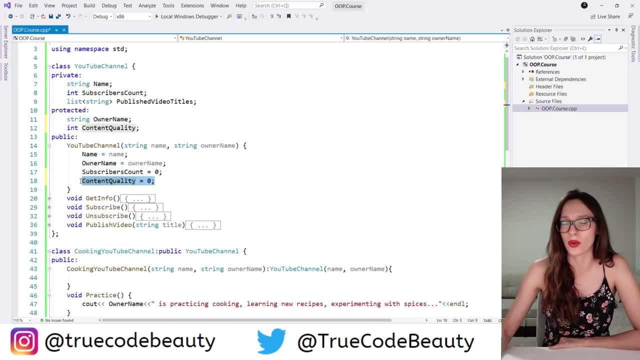 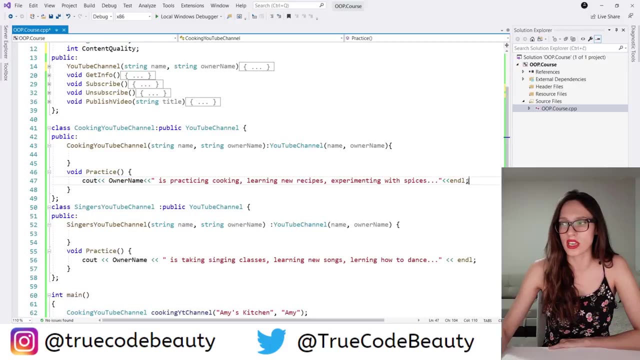 you are going to have zero subscribers and you are going to have a zero knowledge about content quality. So So our current content quality rate- content quality rate- is going to be zero, So let's close that. And then what I want to do here in this practice method is: I want to say each time that you 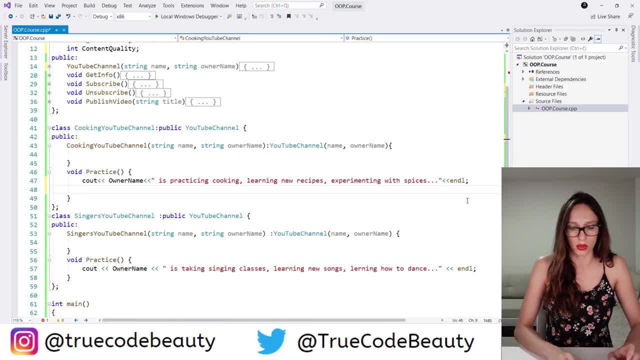 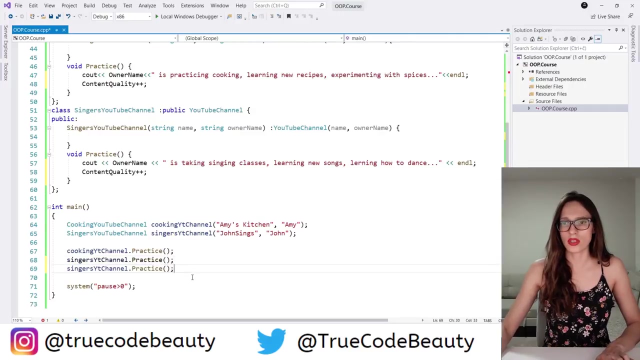 practice. your content quality should increase. So let's increase that variable Content. where is it? Content quality plus plus. So I'm going to increment that content quality And then I'm going to do the same here. So Okay, here, like this: now let's say, for example, that my um, this singer here, john, he's going to practice. 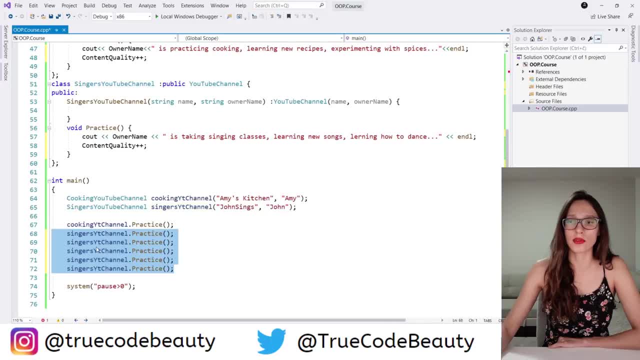 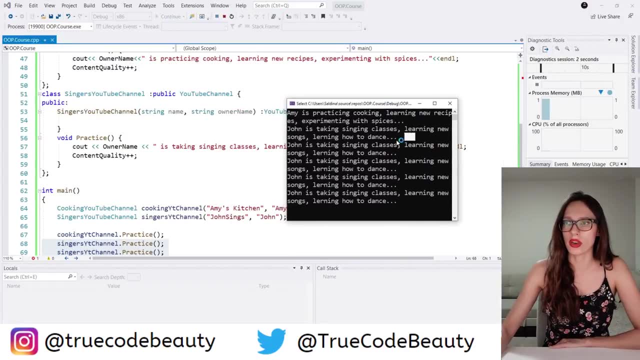 a lot. so he has practiced five times more than amy did. so if i run my program now, you can see that john is practicing and then again and again and again. so he is practicing a lot and amy is not really. so what do i want to do with this? content, quality property, well, 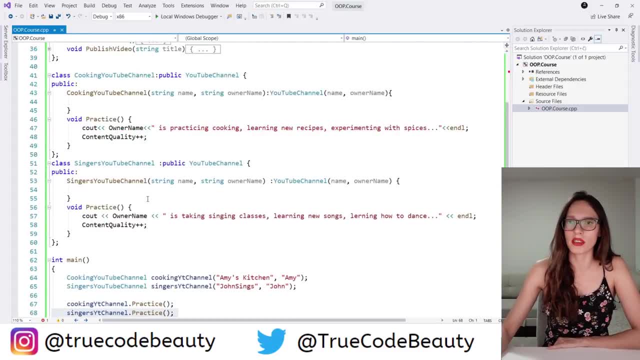 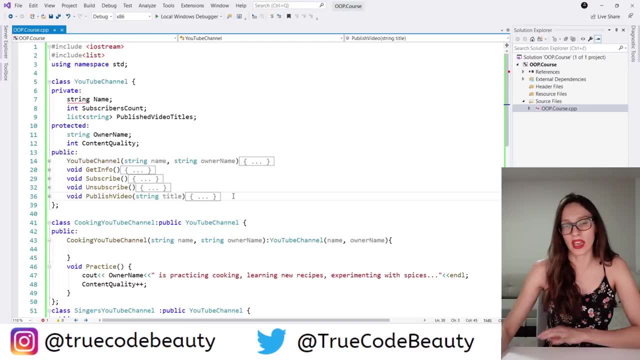 let's say that i want to implement another method, and that method is going to be as well implemented here in this base class, and that method is going to be called, uh, check analytics, because that check analytics method should be available for all youtube channels. so that is not something. 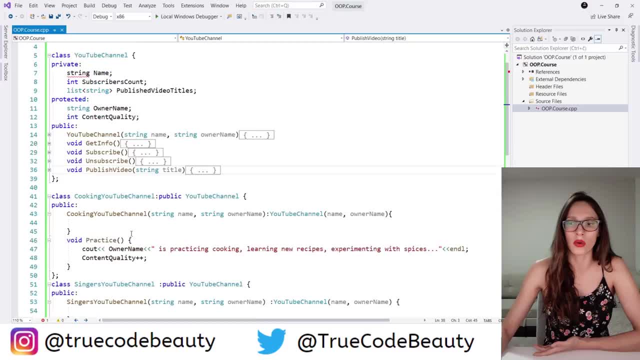 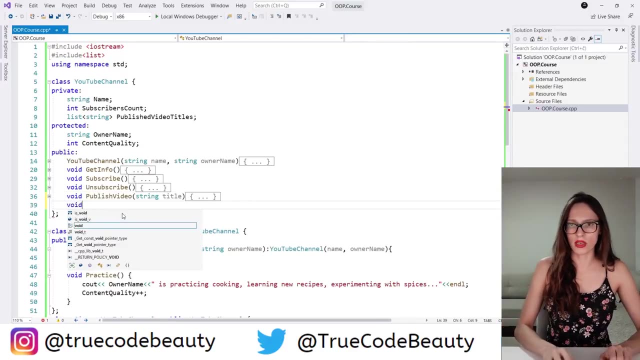 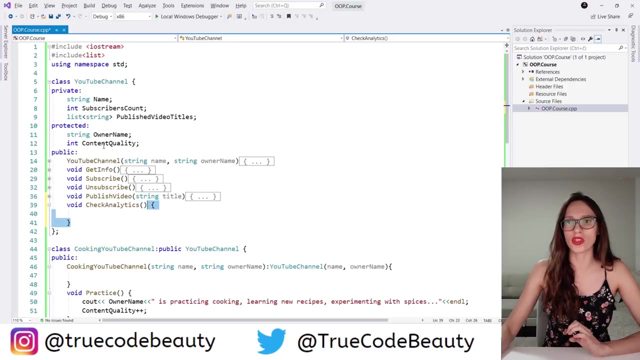 that is specific for this cooking youtube channel only or for this singing youtube channel- so singer youtube channel- but that method should be available for all youtube channels and because of that, i'm going to implement it in this base class. so let's say, void check analytics like this. okay, and now what i want to do in this check analytics method is: i want to use this: 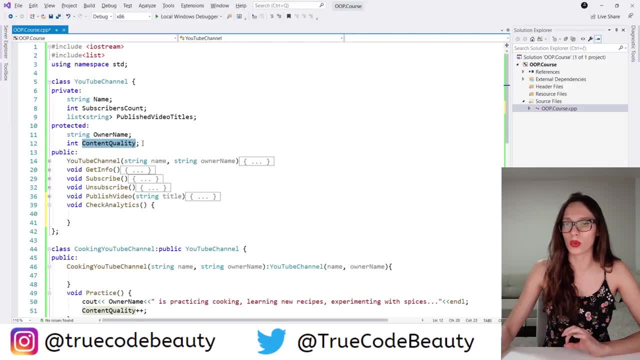 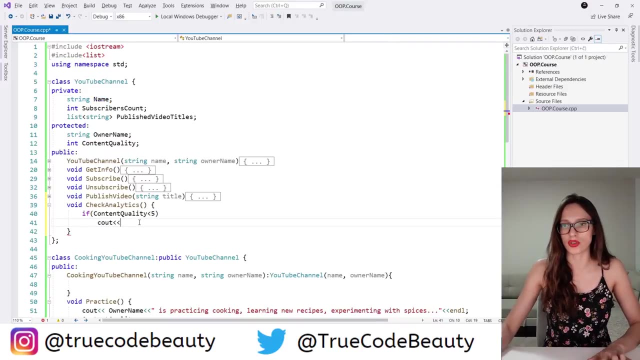 property, this content quality property, in a following way. so i want to say: if content quality is less than five, i want to write out a message to my user. so i want to say c out and then let's write out the name of this youtube channel like this: and then let's add um a message which is going to say: let me copy that. 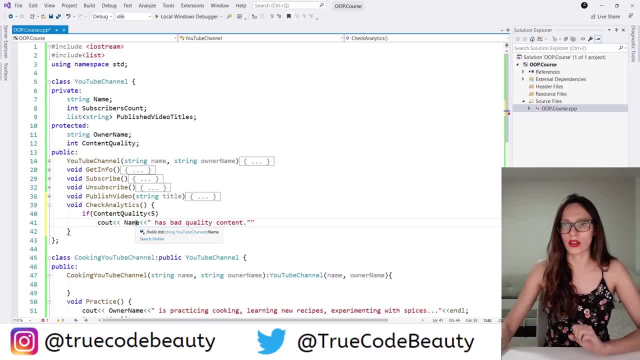 okay, this is going to say that this channel has a bad quality content, because this content quality has a rating, this that is less than five, and let's add n line. and then what is going to happen if this content quality is not, uh, less than five? so if it is, 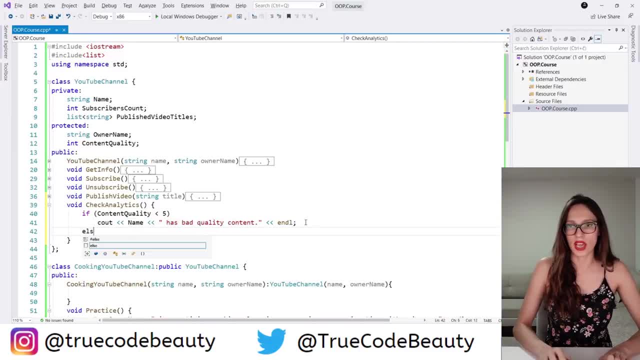 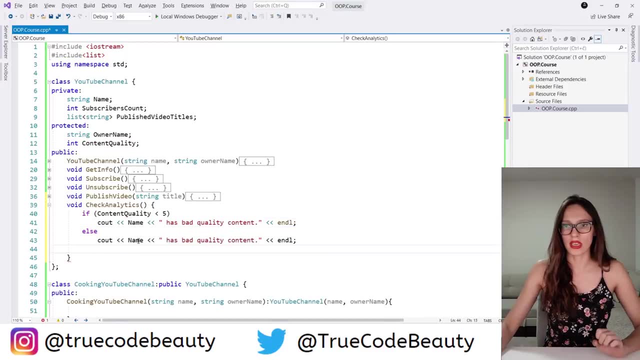 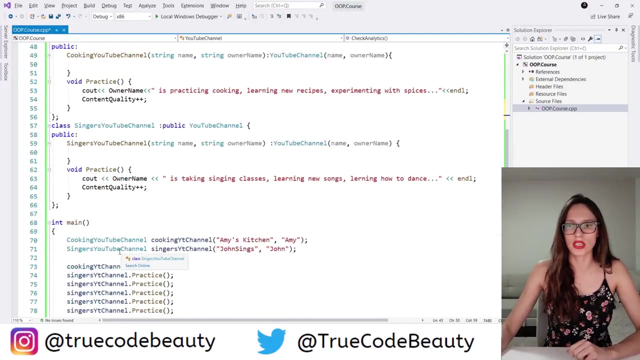 equal to five or greater than five. i'm going to put else block here. and what i want to say here, okay, is that this channel has a good content, great content, actually. okay, like this. now, what am i going to do with this check analytics method? well, i'm going to try to invoke it here, but the way that i want to try to invoke this, 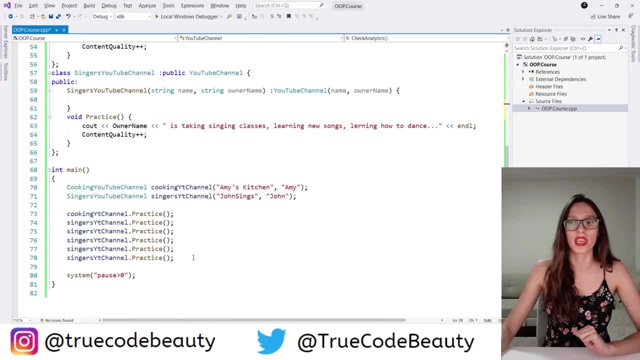 this method that we just implemented is going to be in a following way: so there is one very interesting thing when it comes to polymorphism, and that thing is related to pointers. at this point i haven't made videos about pointers on my channel, but if you're watching this video sometime in the future, then 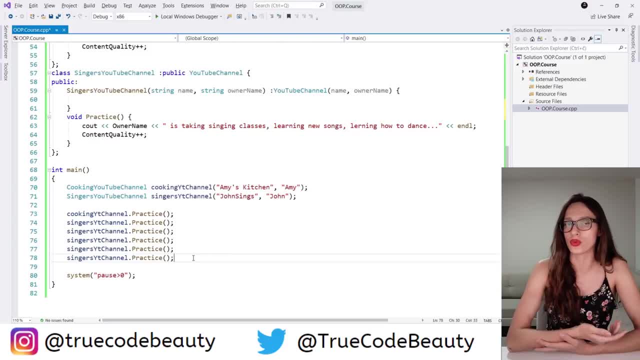 those videos are probably available on my channel, so make sure to look for them on my channel and then in the description of this video as well. so let's create a pointer, and that pointer is going to be a pointer of our base class, so a pointer of type youtube channel. okay, like this, and let's call it youtube one, and what i want to do is: 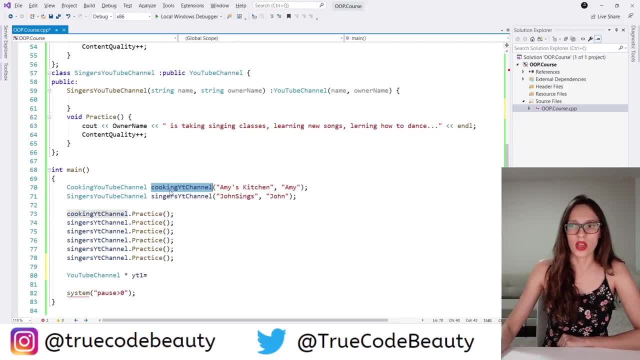 i want to assign to this pointer here address of this cooking youtube channel, and you can do that. you can assign to a pointer of a base class an address of derived class. so i'm going to say here: please this pointer: assign address of this cooking youtube channel class. 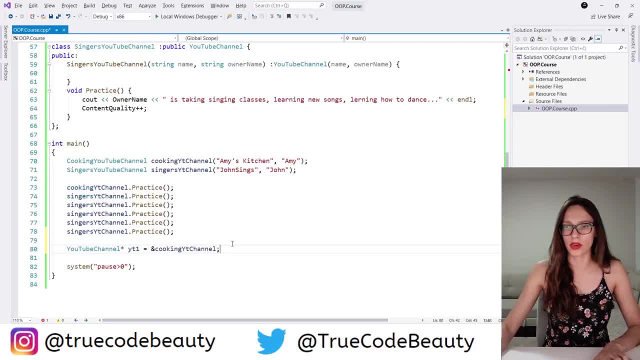 like this, and then what i want to do is i want to create another pointer- let's call it youtube, YouTube2- and then to this YouTube2 pointer I want to assign the address of my singer's YouTube channel like this. So one more time, a pointer of base class can point to a variable of derived. 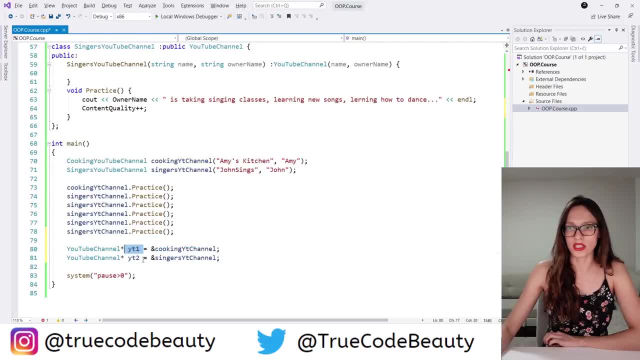 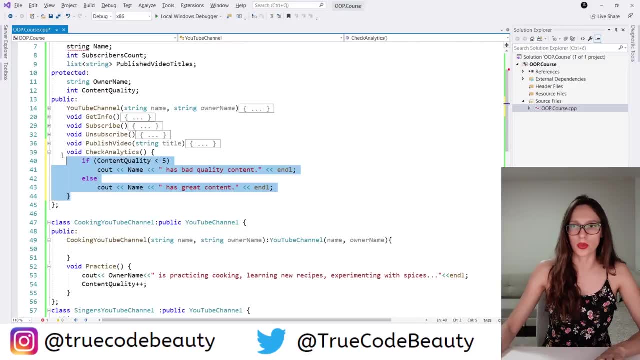 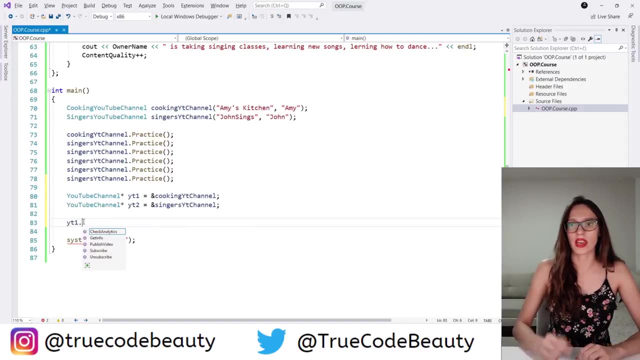 class. Now, what I can do using these pointers is I can invoke method that I have just created, which is this one here. So check analytics. So let's do that. Let's say YouTube, channel 1, and then let's invoke this method. Let's say check analytics, like this: and if you just noticed, 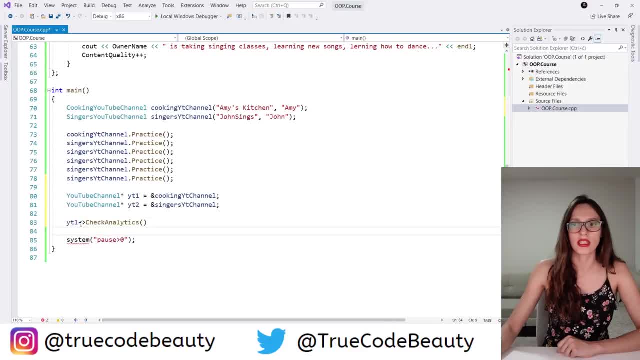 it has changed my dot to this symbol here because this is used when you want to invoke methods using pointers. So I'm going to copy this again for my second YouTube channel like this. and now, if I running run my program, as you can see, our John has been practicing a lot, and then Amy. 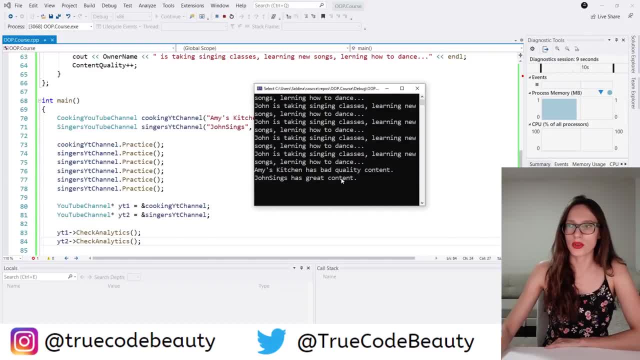 has been practicing only one time. so here, after I have invoked these two methods, this first method says that Amy's kitchen has bad quality content because she hasn't been practicing enough. and then, after this YouTube channel 2 check analytics, you can see that it writes out this message that 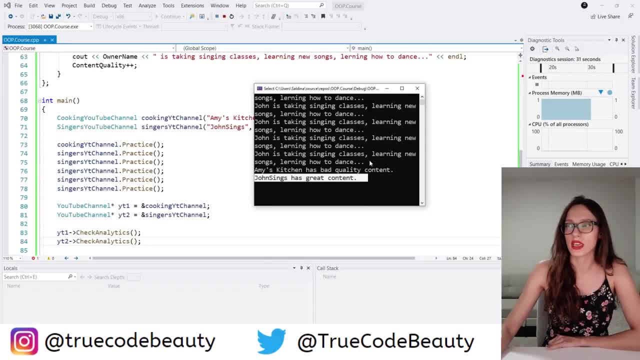 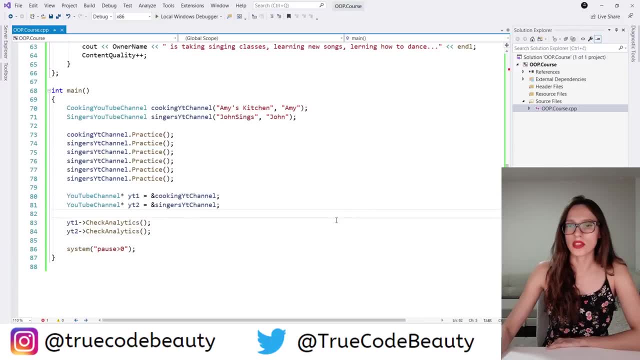 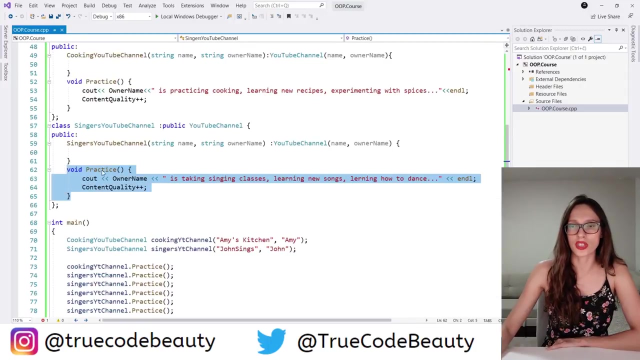 John Singh channel has great content because he has been practicing a lot, as you can see here. ok, so here we have used polymorphism in order to implement this practice method in our cooking youtube channel and then in our singers youtube channel. so implementation of our singers youtube channel. 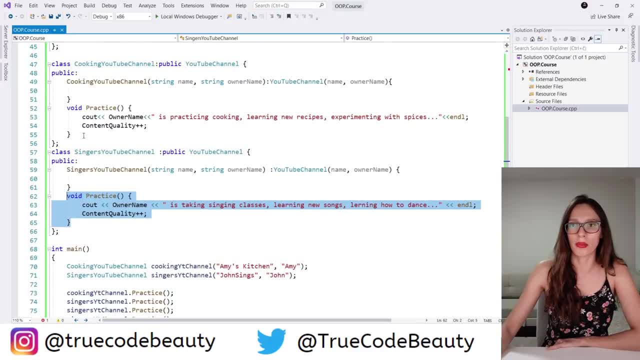 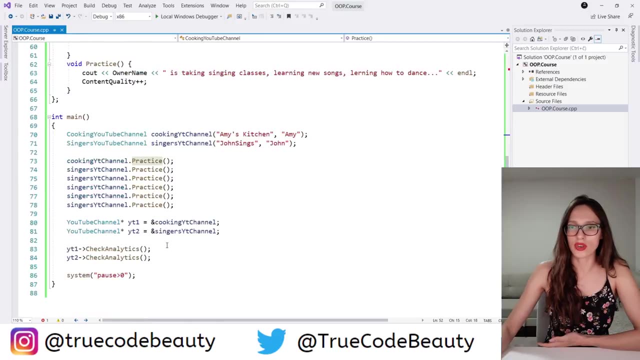 practice method is here. and then for our cooking youtube channel our practice method looks like this, and we have done that thanks to the polymorphism. so different implementations, but the same method name. and then i have demonstrated here how you can use pointers to point to an object of derived class and you can store that in a pointer of base class. and then we